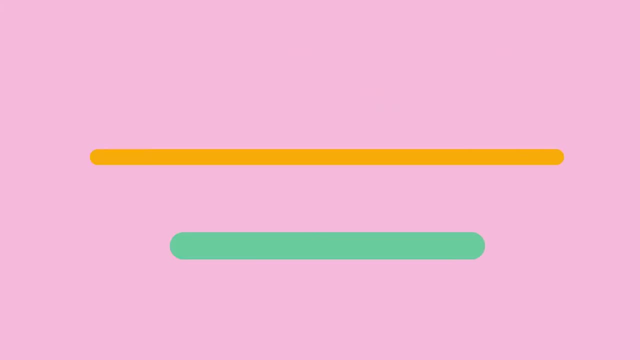 So why does charge flow and therefore current? For electrons to flow, we need two things: One, a source of potential difference, which is also known as voltage. This provides the pressure that makes the current flow. And two, a complete circuit. The circuit must have no breaks in it to 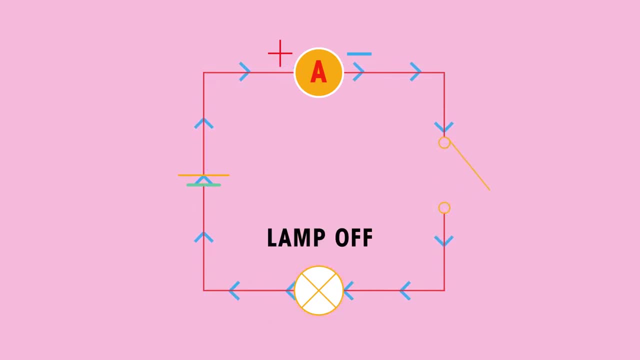 be complete. If there are breaks, then no current can flow. In fact, that's how a switch works. To switch an appliance off, we create a break in the circuit to prevent the current from flowing. To switch an appliance on, we close the switch, which completes the circuit and so allows the 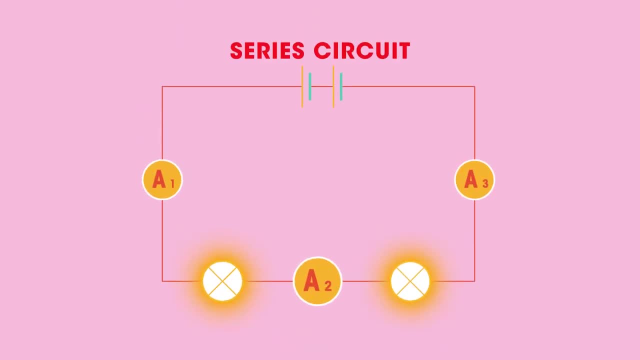 current to flow In a series circuit, so all components are in a line, one after the other. all the electrons travel through every component and wire. as they travel through the circuit, All the electrons experience the same resistance, and so they all move at the same rate. This 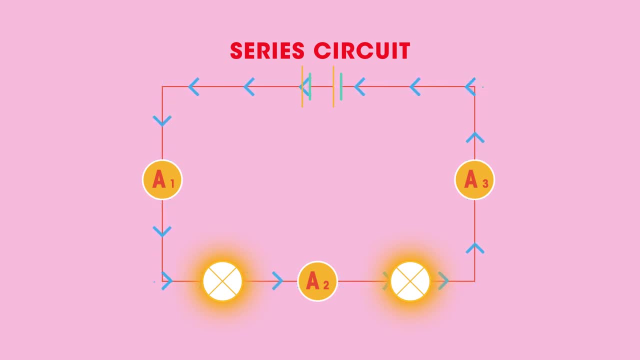 means that in the series circuit, the readings on all three elements are the same. The readings on all three ammeters will be the same: A1 equals A2, which equals A3. This is not true, however, for parallel circuits. In parallel circuits, the current is shared between the different branches of the 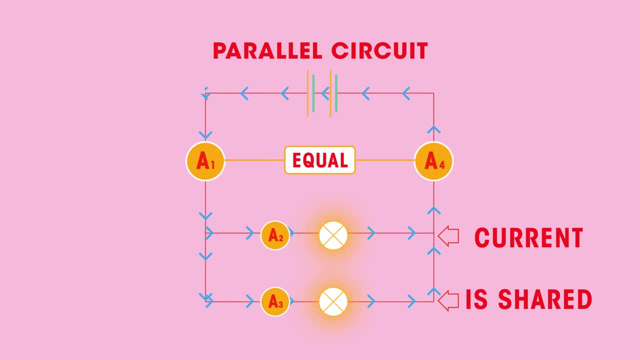 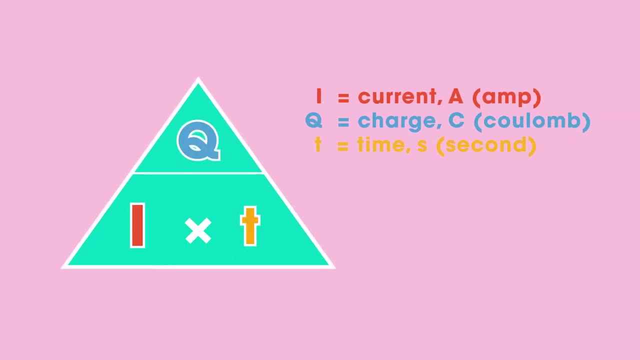 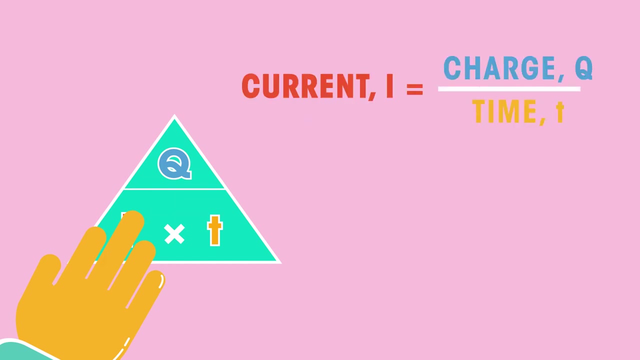 circuit. So A1 equals A4, but A1 equals A2 plus A3, which equals A4.. To calculate the current in a circuit we can use this formula To charge divided by time. It makes sense that current is charged divided by time because current 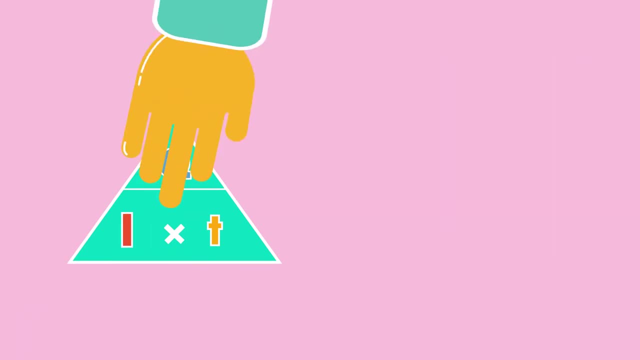 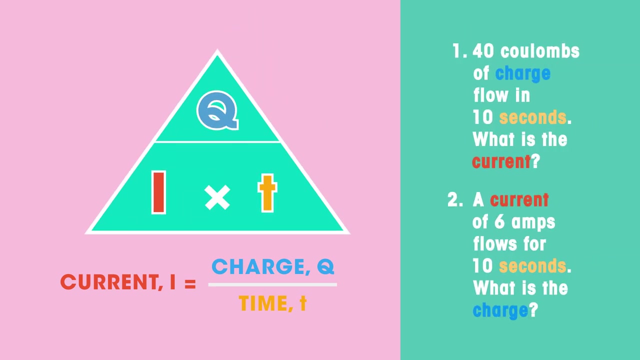 is the rate of flow of charge, Or I actually find it easier to remember quit QIT. Charge equals current times, time. So using the relationship between charge current and time, can you answer these questions? Pause the video and work it out.